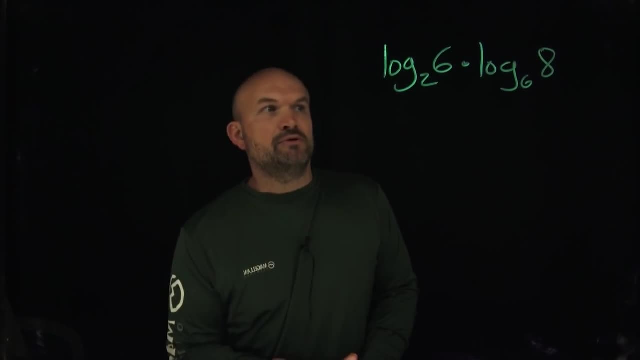 rules of logarithms or the properties of logarithms, right, And I think one of the first things we always do in class, like when we're giving you the notes, you know as a teacher, like that, here's all your notes- like one thing I always like tell my students like you can. 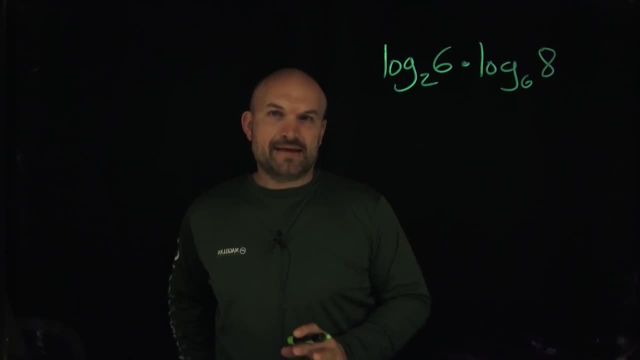 only apply the properties of logarithms when the bases are the same. you know that's especially when we're looking at the product and the- you know quotient properties and stuff like that. You know one thing I kind of recognize with this one, or at least when I'm looking. 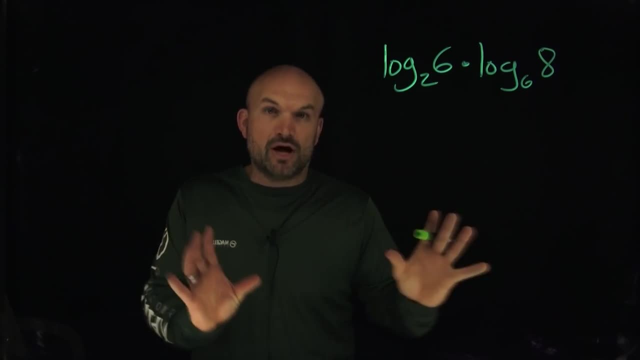 at this. this isn't like the product like, remember the product represents. like two separate logarithms that are separated by addition, right? Then we multiply the arguments again only when the bases are the same. Now again I have that red flag. like the bases are not, 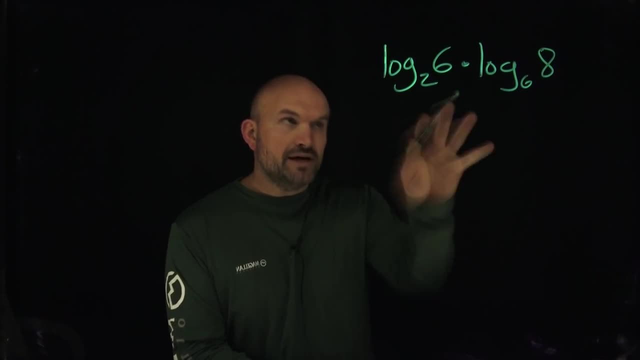 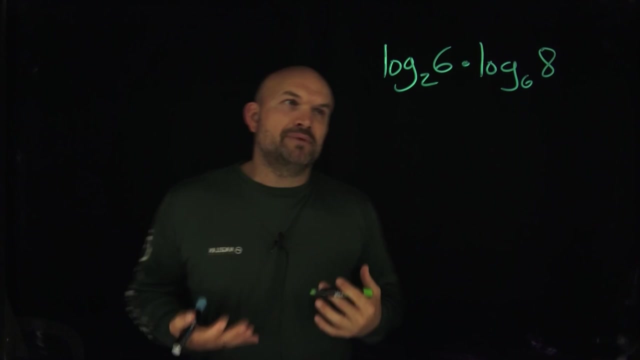 the same right, So I can't use my typical properties of logarithms. But the other thing that's interesting about this problem is I'm actually not adding the two logarithms right. It's already multiplied, So I couldn't even use the product property of logarithms anyways. 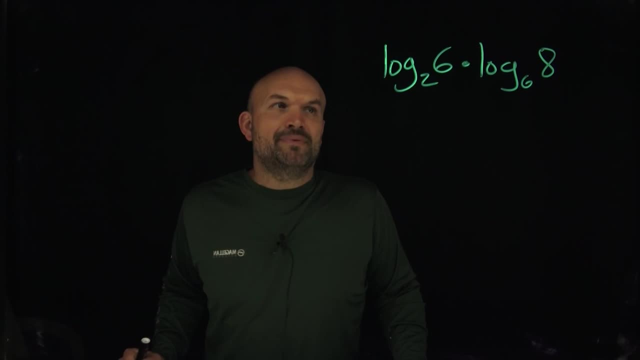 in this case, Like I'm already kind of using the product property of logarithms, right, So I'm already kind of stuck. So one of the one of the properties though that I think a lot of times gets overlooked- and I'm victim of this as a teacher as well- It's like one of the last. 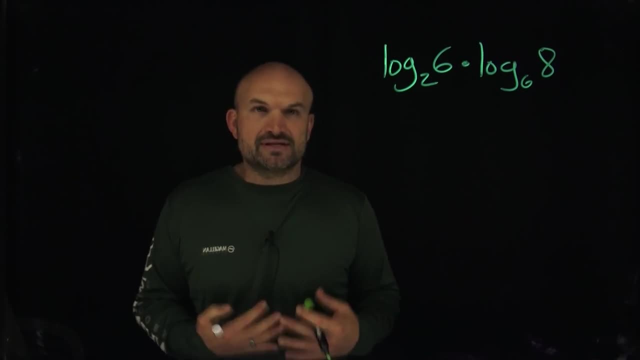 problems we talk about And- and it's usually one of those properties We just kind of relate to students. I'm like, oh yeah, if, like you, don't have a calculator, you can use it. But a lot of times we don't investigate problems where it is required to be able to use And 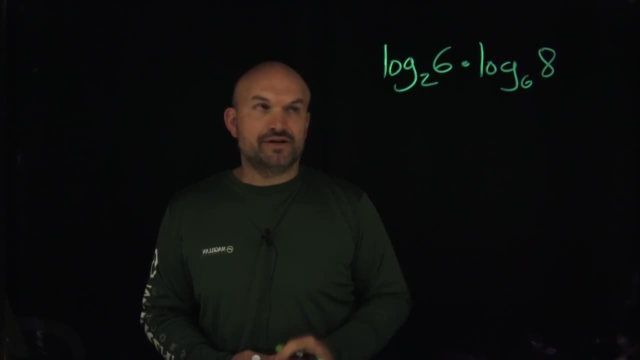 that is going to be the change of base formula. So we recognize there's really not much I can do here. but one thing I can do is use the change of base formula. Now, when I personally like to use a change of base formula, I always like to use logarithms. And again, just a. 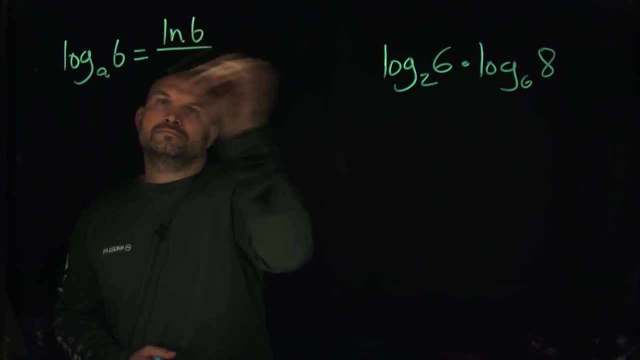 quick reminder: the change of base formula. It just looks like this: Okay, So basically what I'm doing is, if I have a logarithm with the base A of B, I can just rewrite this as the logarithm of the argument in this case. 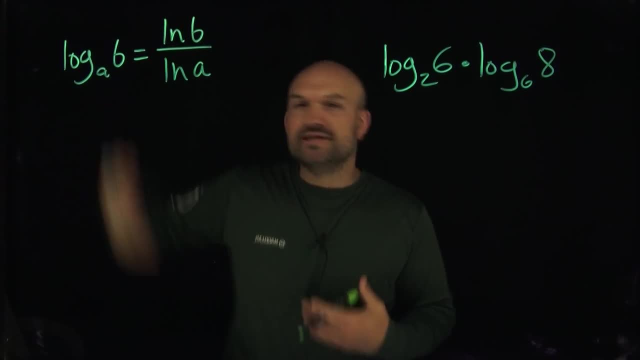 B, divided by the logarithm of the argument from the original base. Now I'm using the natural logarithms, but a lot of times you know you can use base 10 or in reality you can use any base that you want to. It doesn't really matter, I always like to use logarithms. 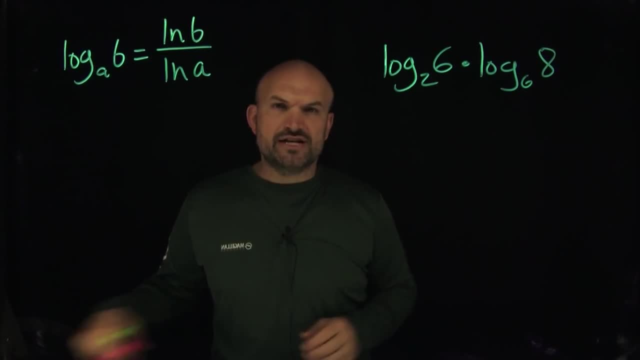 I don't know why. It's just it's kind of been my habit. So let's go and use the change of base formula. Let's see in this problem if that's going to help us, like I don't know. 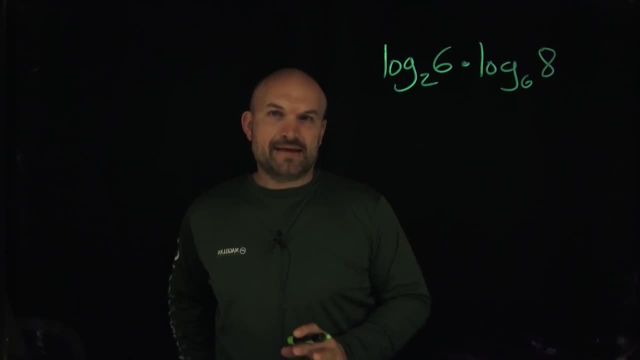 only apply the properties of logarithms when the bases are the same. you know that's especially when we're looking at the product and the- you know quotient properties and stuff like that. You know one thing I kind of recognize with this one, or at least when I'm looking. 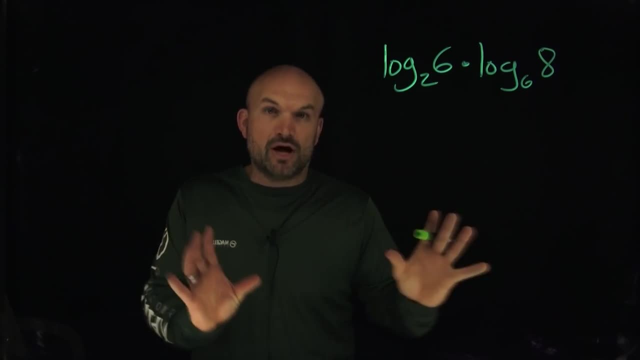 at this. this isn't like the product like, remember the product represents. like two separate logarithms that are separate by addition. right, then we multiply the arguments again only when the bases are the same. Now again, I have that red flag. like the bases are not, 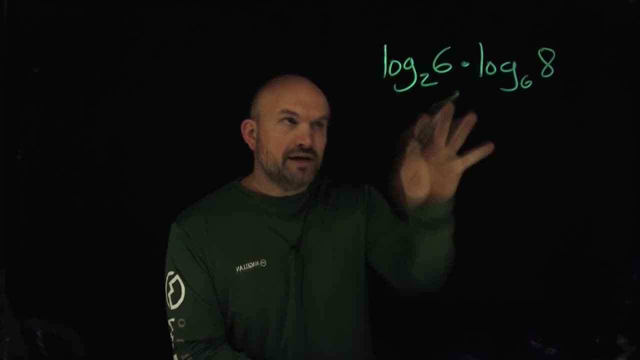 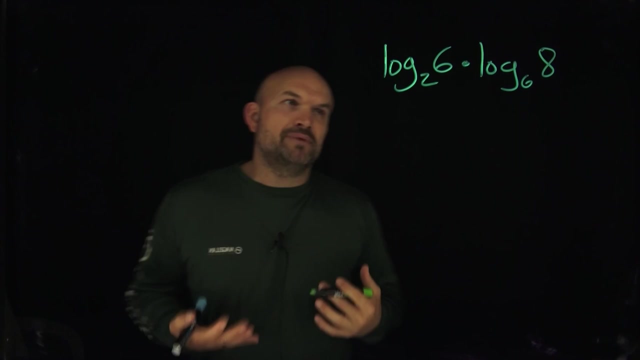 the same right, So I can't use my typical properties of logarithms. But the other thing that's interesting about this problem is I'm actually not adding the two logarithms right, it's already multiplied, So I couldn't even use the product property of logarithms. Anyways, 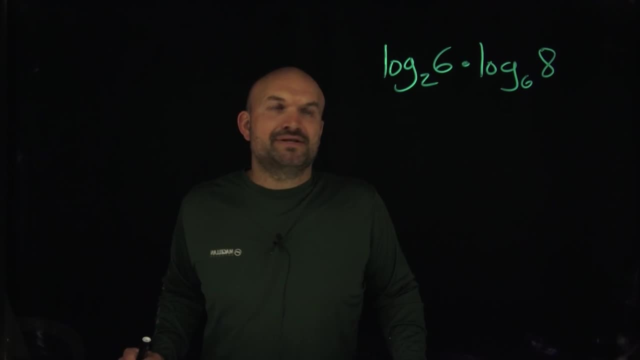 in this case, like I'm already kind of kind of stuck. So one of the one of the properties, though, that I think a lot of times gets overlooked- and I'm victim of this as a teacher as well- It's like one of the last problems we talked. 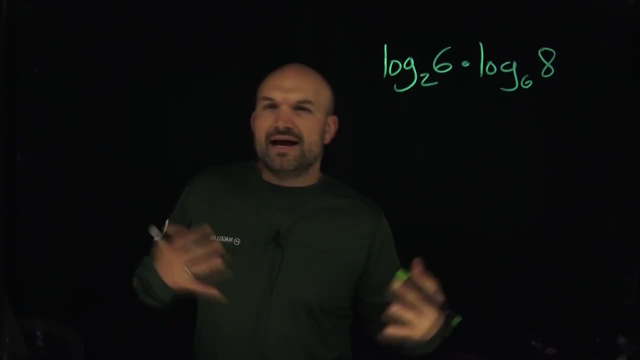 about And- and it's usually one of those properties we just kind of relate to students. I'm like, Oh yeah, like you don't have a calculator, you can use it, But a lot of times we don't investigate problems where it is required to be able to use and that is going to be. 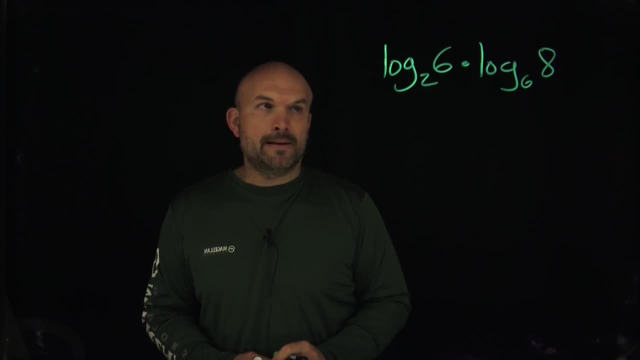 the change of base formula. So we recognize there's really not much I can do here. But one thing I can do is use the change base formula. Now, when I personally like to use a change base formula, I always like to use logarithms. And again, just a quick reminder. 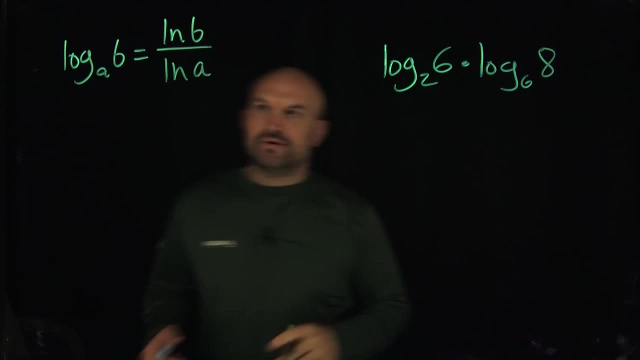 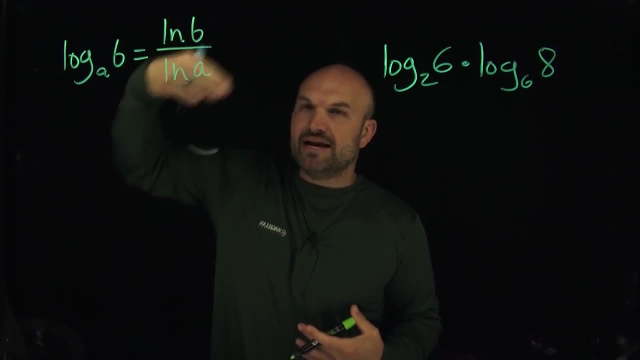 the change base formula just looks like this: Okay, so basically what I'm doing is, if I have a logarithm with the base A of B, I can just rewrite this as the logarithm of the argument, in this case B, divided by the logarithm of the argument from the original base. Now I'm using the. 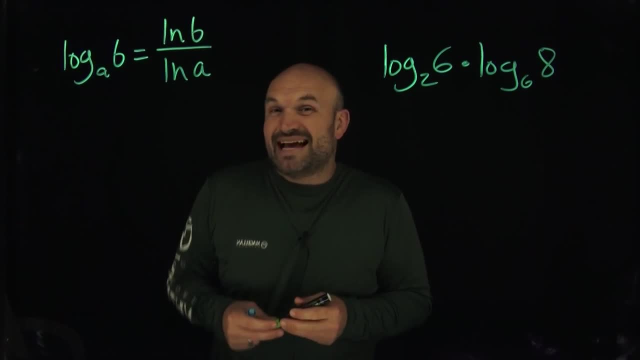 natural logarithms, But a lot of times you know you can use base 10.. Or in reality you can use any base that you want to. it doesn't really matter. I always like to use logarithms. I don't know why, it's just it's kind of been my habit, So let's go and use. 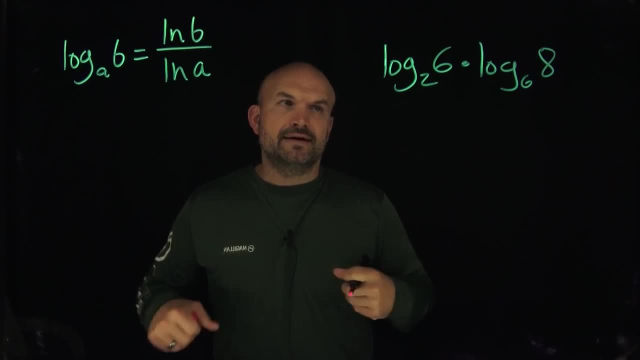 the change base formula. Let's see in this problem if that's going to help us, like I don't know- simplify this at all. So what I'm gonna do is let's go ahead and apply change base form for both of them And remember I got to keep this multiplication here, Okay, 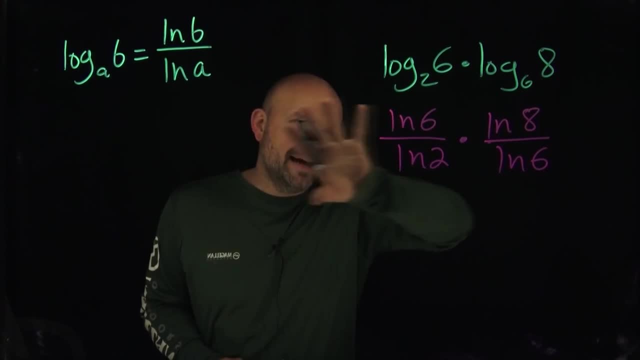 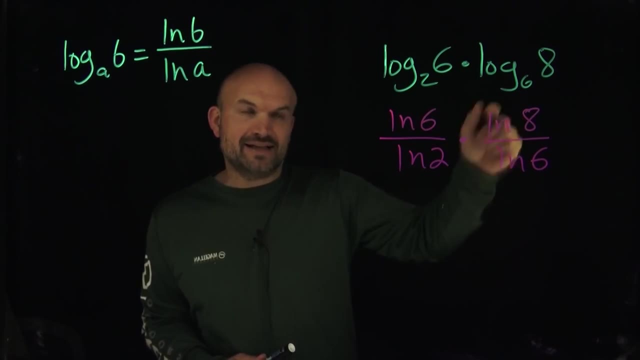 so now, hopefully you recognize that, ah, something interesting is happening, Like as I'm multiplying these- or at least everything is separated by multiplication- I noticed that I have the same expression, ln of six and ln of six, in the numerator as well as in the denominator. 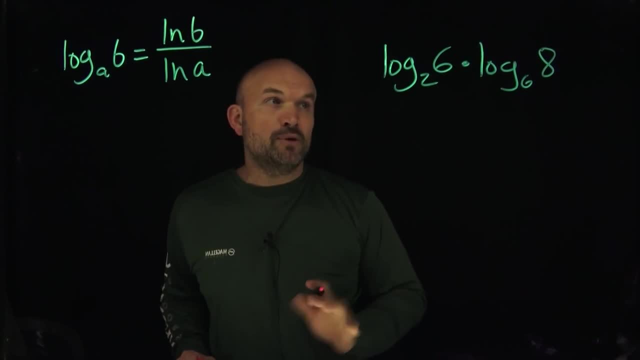 simplify this at all. So what I'm going to do is: let's go ahead and apply the change of base formula for both of them And remember we've got to keep this multiplication here. Okay, So now, hopefully you recognize that. ah, something interesting. 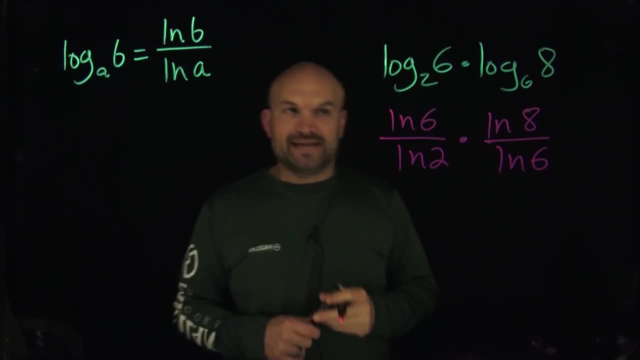 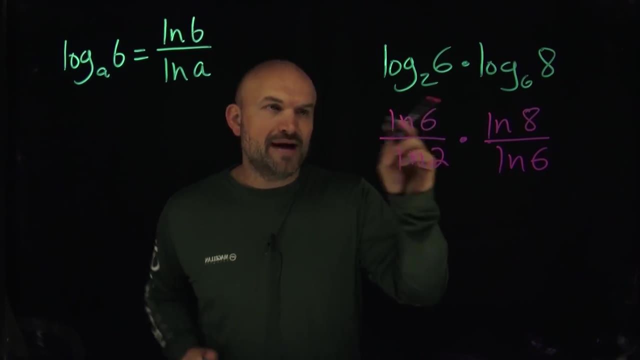 is happening Like as I'm multiplying these- or at least everything is separated by multiplication- I noticed that I have the same expression, ln of six and ln of six, in the numerator as well as in the denominator, So now I can use my division property and divide those out. 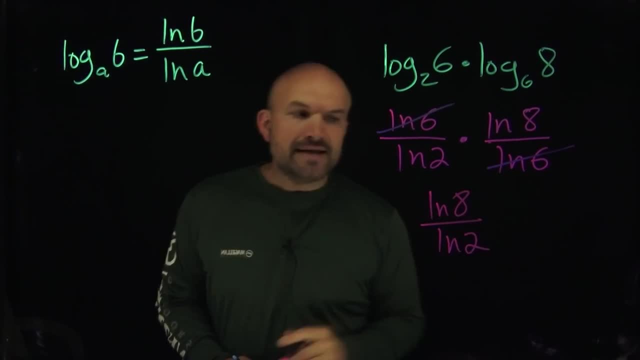 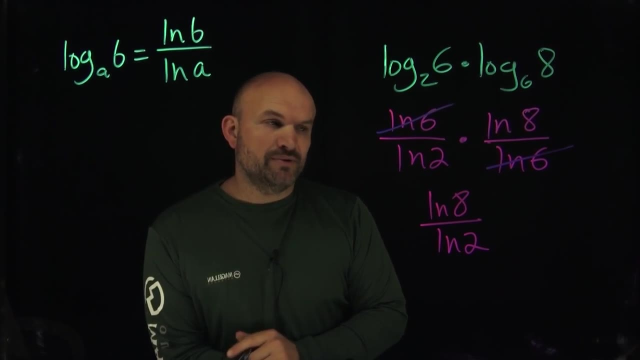 That's now going to leave me with a ln of eight over ln of two. Now, in this case, you still might be stuck and you might be saying like well, I don't know what to do from here. Like still kind of suck, Like what do you do? So one thing that you could do is look. 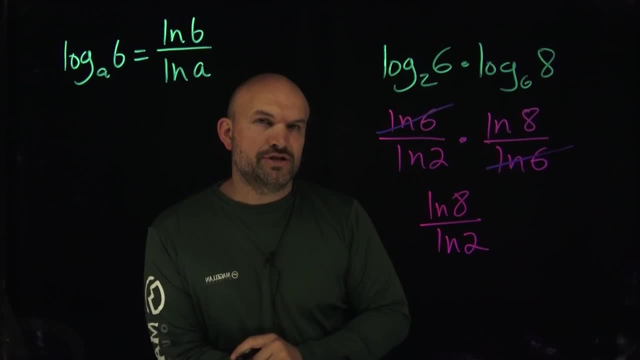 at the arguments and recognize that there's a relationship between an eight and a two right, And that relationship here is that eight can be rewritten as a two cubed. Now, why would I want to go ahead and do that? And you might say, well, I don't know. but 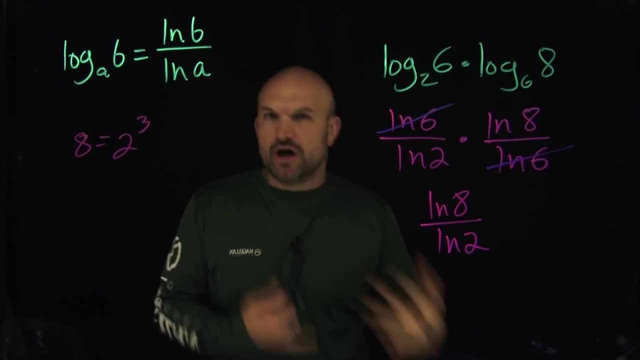 again. I see that relationship. So a lot of times in mathematics when we're trying to solve or trying to do something, we get stuck. you know like you might've thought about. you might not have thought about the change of base formula here, but like one thing I 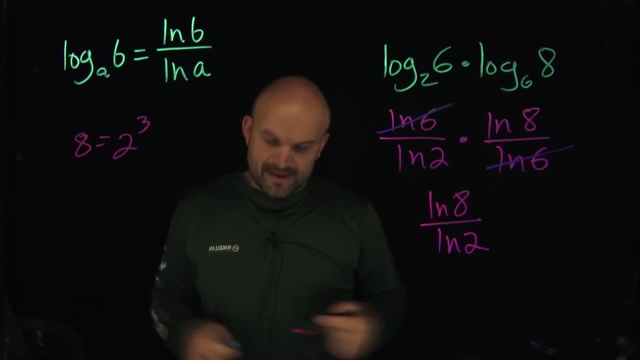 would you know, advise you to start looking at is like think about, like well, maybe it's not the right way, Maybe it's not, but like try things right And be okay If you're getting it wrong, like it's all a part that you know discovery and trying to see like 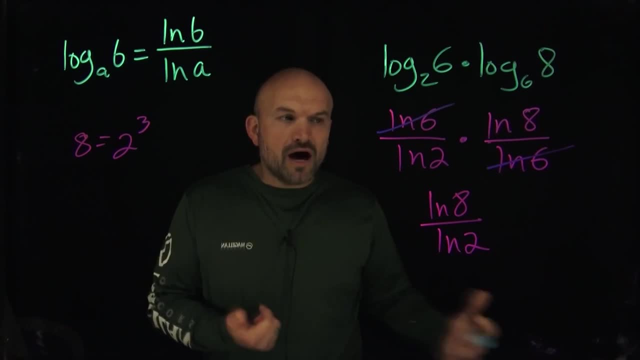 you know, can I use this? You know, as long as you're not violating any mathematical laws like, feel free to try things and see if they work. Sometimes you might have found out a better way than what your teacher was teaching you, right, Or at least a way that makes more. 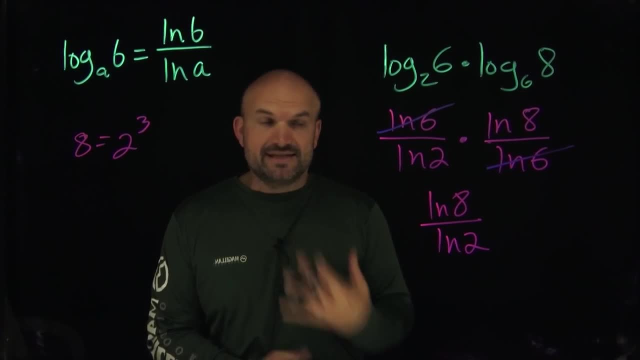 sense to you than what maybe your teacher was teaching. And I know as a teacher I found that many, many times like I might explain something and the students like why didn't you do it this way? It's much easier. And I'm like, oh yeah, you're right, That was. 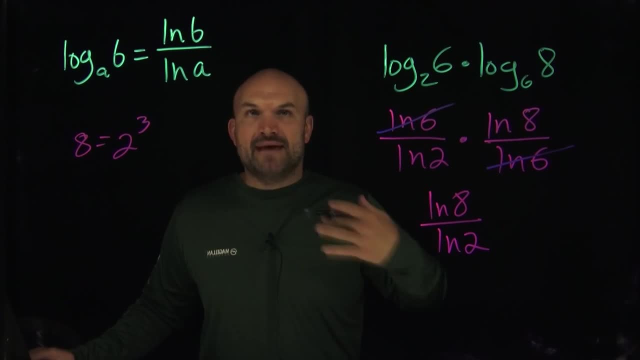 a much better way. Um, and then the other thing that I would say is, like you know, if you're trying to solve a problem, you know it's just the way that I saw the problem and you know through my experience, but you know that might not be the best or the easiest for any of you. 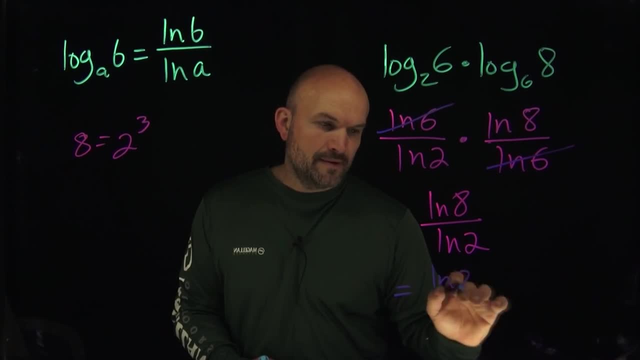 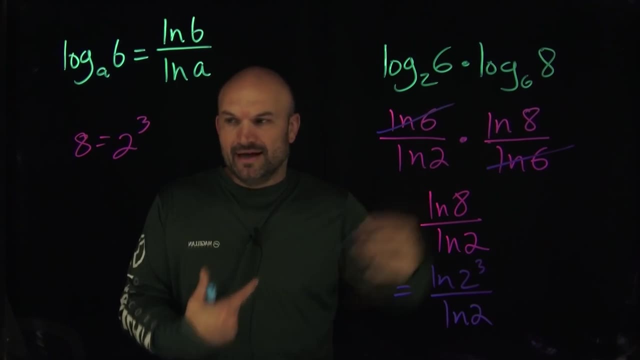 If we go ahead and rewrite this, then what I'll have now is a ln of two cubed all over an ln of two. So now what this record, what this triggers to me, is the product property- And remember, the product property of a logarithm basically states: if you have like, if you. 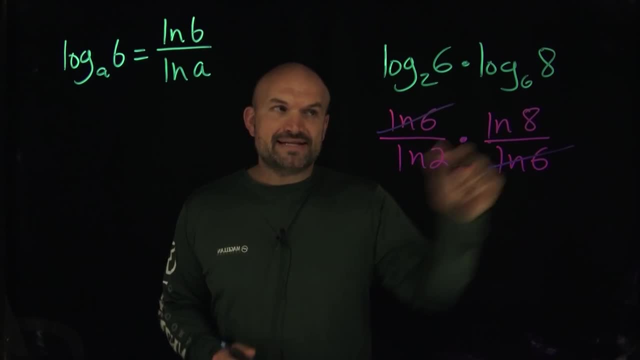 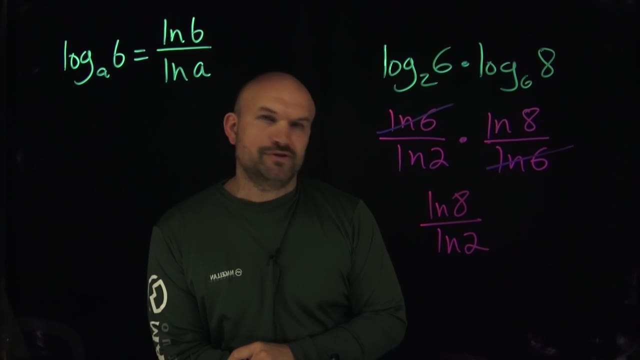 So now I can use my division property and divide those out. That's now going to leave me with a ln of eight over ln of two. Now, in this case you still might be stuck And you might be saying like, well, I don't know what to do from here. 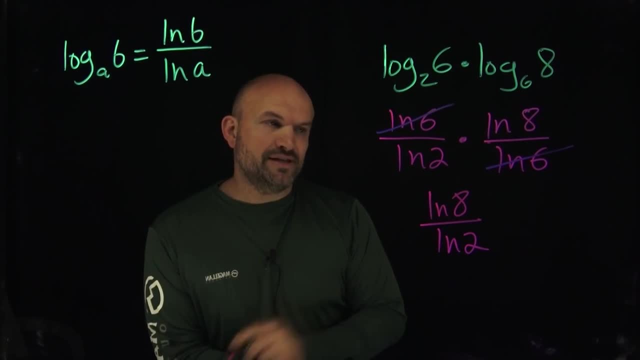 Like still kind of suck. Like what do you do? So one thing that you could do is look at the arguments and recognize that there's a relationship between an eight and a two right, And that relationship here is that eight can be rewritten as a two cubed. Now, 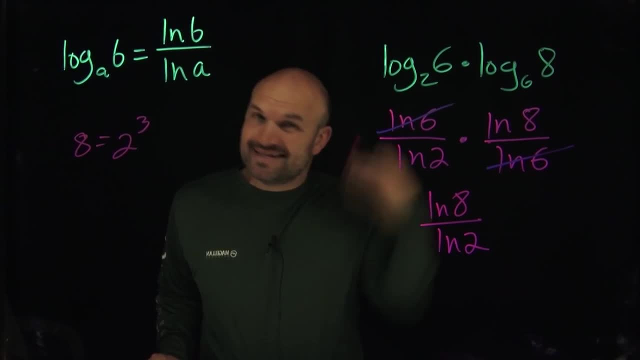 why would I want to go ahead and do that? And you might say, well, I don't know. But again, I see that relationship. So a lot of times in mathematics, when we're trying to solve or trying to do something, we get stuck. You know, like you might have thought about. 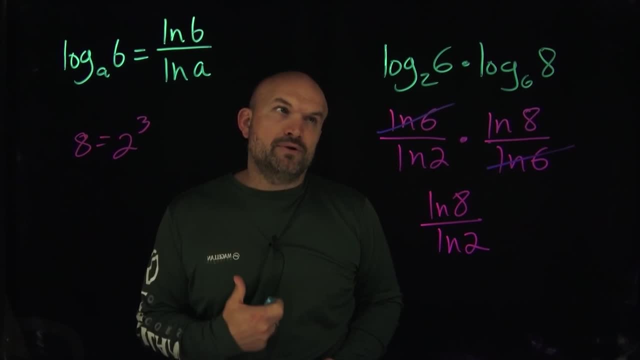 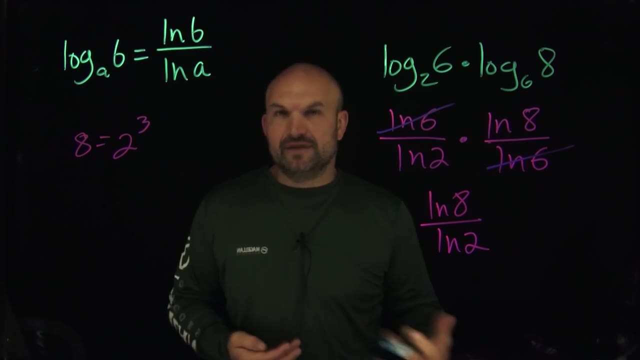 you might not have thought about the change of base formula here, But like one thing I would, you know, advise you to start looking at is like think about, like well, maybe it's not the right answer, Maybe it's not, but like try things right And be okay if you're getting it wrong. Like 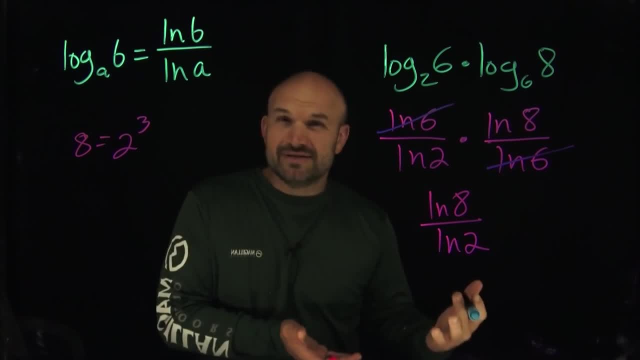 it's all a part that you know: discovery and trying to see. like you know, can I use this, You know, as long as you're not violating any mathematical laws like, feel free to try things and see if they work. Sometimes you might have found out a better way than what. 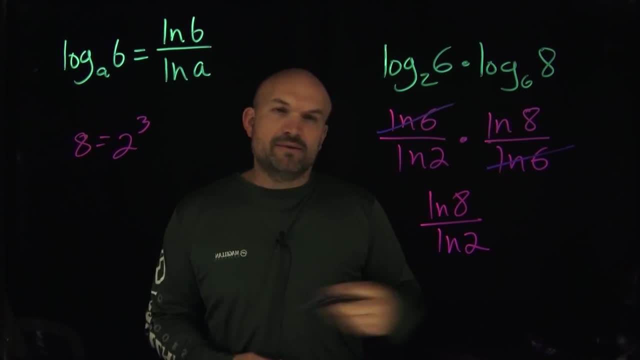 your teacher was teaching you right, Or at least a way that makes more sense to you than what maybe your teacher was teaching. And I know as a teacher I found that many, many times like I might explain something and the students like why don't you do it this? 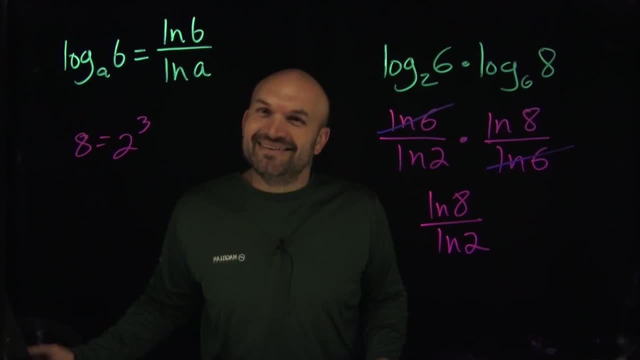 way It's much easier And I'm like, oh yeah, you're right, That was a much better way. You know it's just the way that I saw the problem and you know through my experience. but you know that might not be the best or the easiest for any of you If we go ahead. 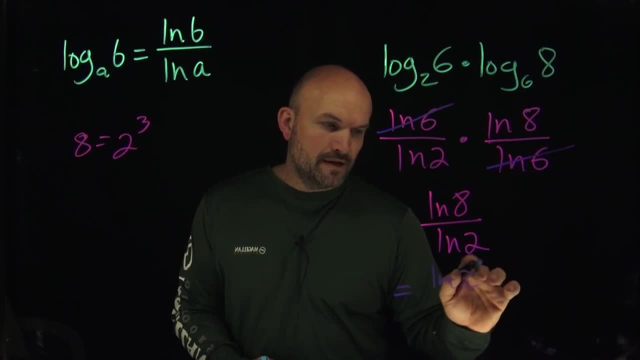 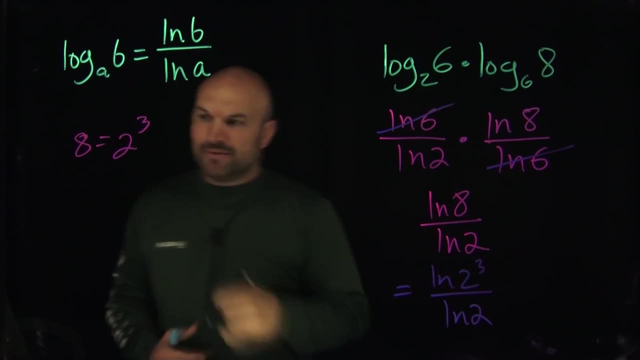 and rewrite this, then what I'll have now is a ln of two cubed all over ln of two. So now what this triggers to me is the product property. And remember, the product property of logarithm basically states: if you have like, if you have a logarithm, base A of B, 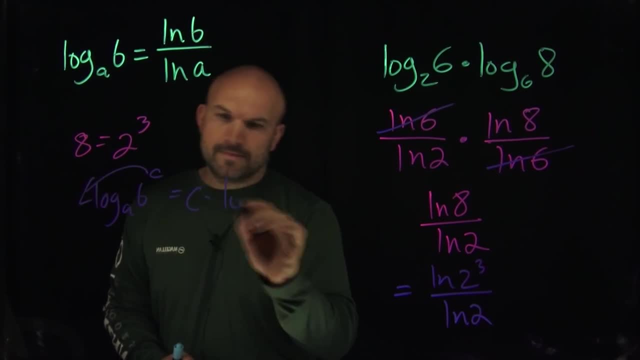 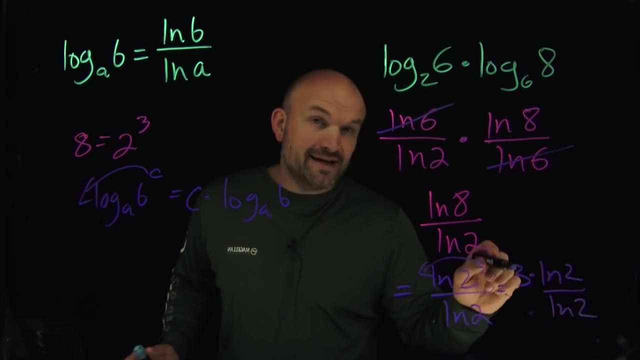 raised to the C power, I can take the C out in front. Now I can just rewrite this: a C times the logarithm base of base A of B, So I can take this 3.. I now have a 3 times ln of 2 divided by ln of 2.. 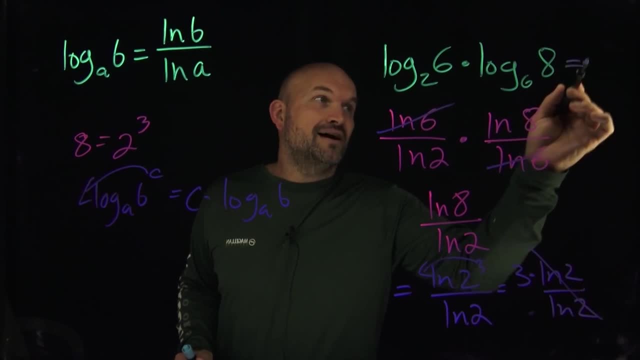 Well, those are going to divide out, leaving me with a final answer, ladies and gentlemen, of just a 3.. Now you know how to use the change of base formula. In the next video, we're going to expand them on this. I'm using the change. of base formula as a power. I'll see you there.